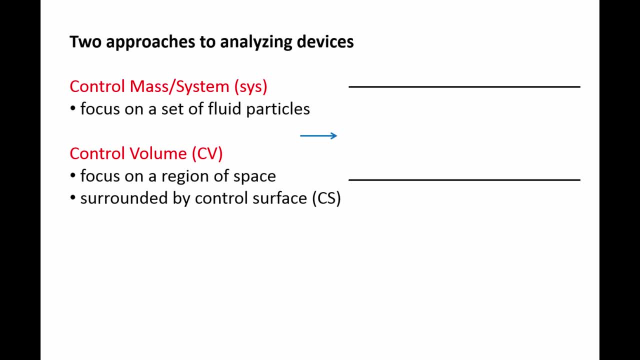 To help illustrate the difference between the system and control volume approaches, let's take a look at fluid flowing through a pipe. The section of pipe we wish to analyze is outlined by red dashed lines. At time, t1,, a specific amount of mass highlighted in pink, occupies the section of pipe. 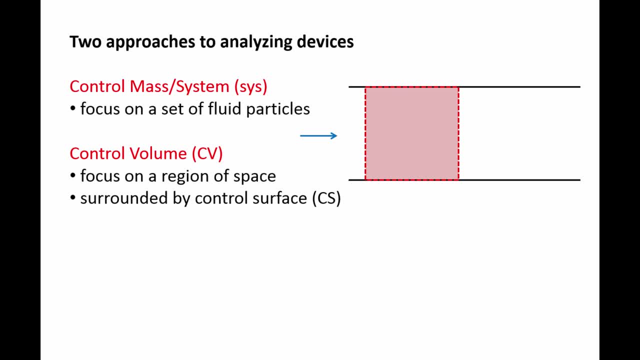 This mass is called a system. The control surface is marked by the red dashed lines and the control volume is inside the control surface. So initially both the system and control volume occupy the same region of space. At a future time t2, the control volume and control surface stay in place, but some of 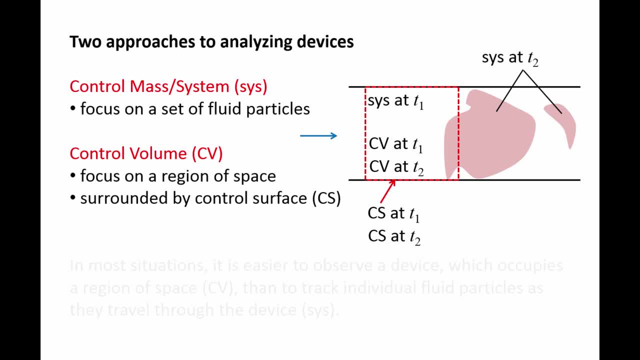 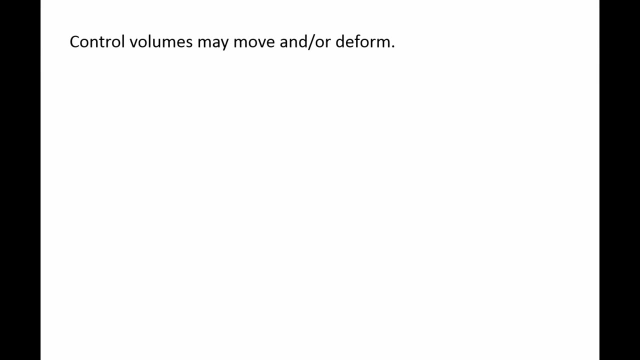 the system has flowed out of the control volume. When analyzing a device, it is usually much easier to observe the region of space occupied by the device rather than track the individual particles as they travel through the device. Although many devices are fixed in place and rigid, such as the pipe we just discussed, 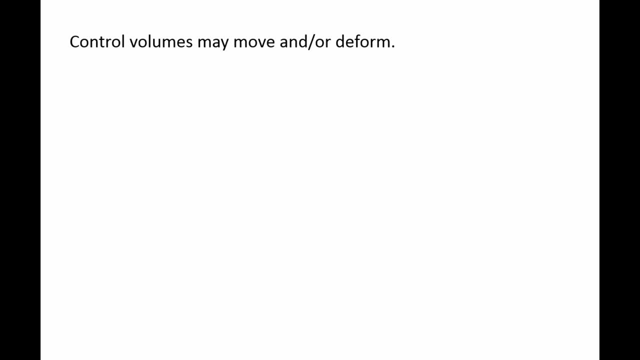 that is not the case for all devices. Sometimes it is necessary to have a control volume that moves or deforms. For example, a jet engine is filled with air, fuel and exhaust gases at time. t1.. The control volume is the region of space occupied by the jet engine and outlined by 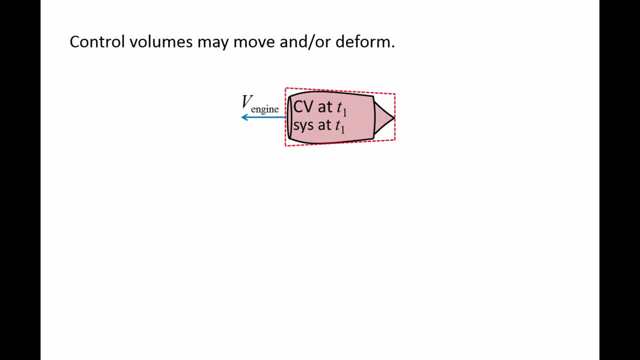 the red dashed lines, The system is the pink shaded area. At time t1,, the control volume and system occupy the same region of space. At a later time, t2,, the control volume has traveled to the left, while the system has been expelled to the right. 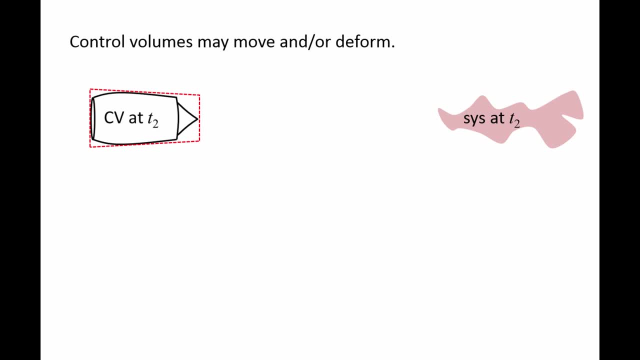 In this case the control volume has moved but not deformed. On the bottom of the screen we have an example where the control volume moves and deforms. A balloon is initially filled with air at time t1. The control volume is outlined by the surface of the balloon and the system is shaded in pink. 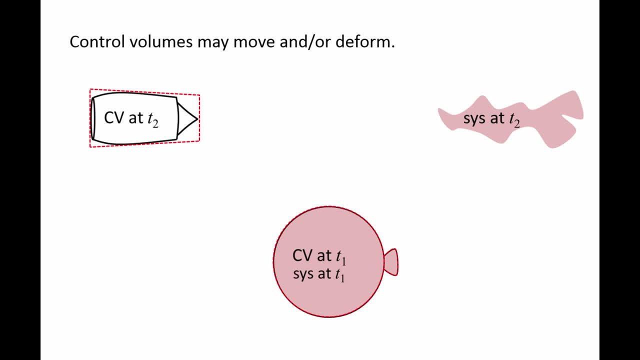 At this time, both the control volume and system occupy the same region of space. Air is allowed to escape and at a future time, t2,. the control volume has moved to the left and become smaller, while some of the system has left the balloon.